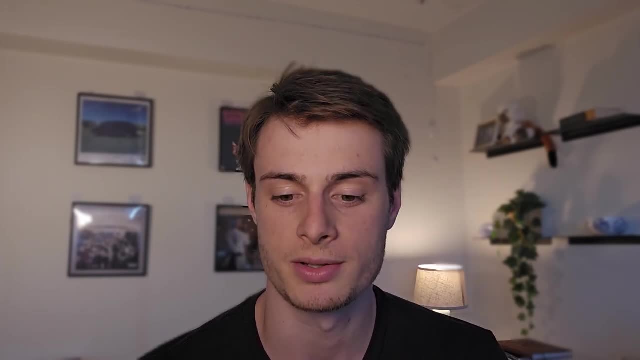 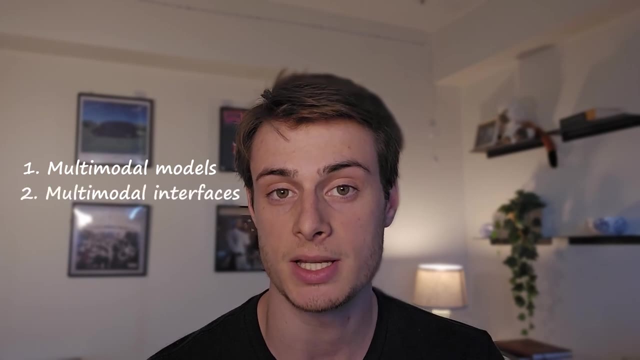 Hey everyone. in this video we're going to talk about how multimodal AI works. First we'll talk about how text-to-image models like DALI work to get an understanding of multimodality in general, and then we'll talk about how interfaces like ChatGPT are able to. 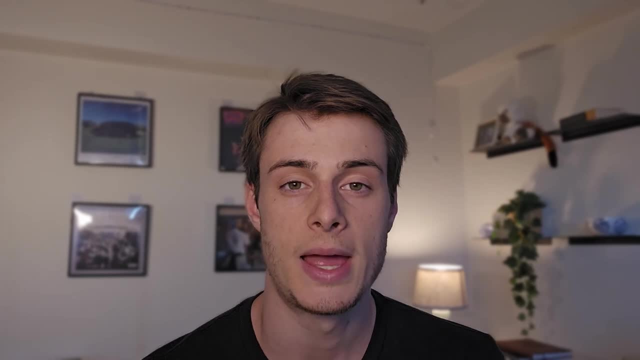 both take in and generate text, audio and images At their core. multimodal models tend to share similar operating principles, regardless of the particular modalities considered, So let's start with text-to-image models. like DALI, Modern image models are generally built. 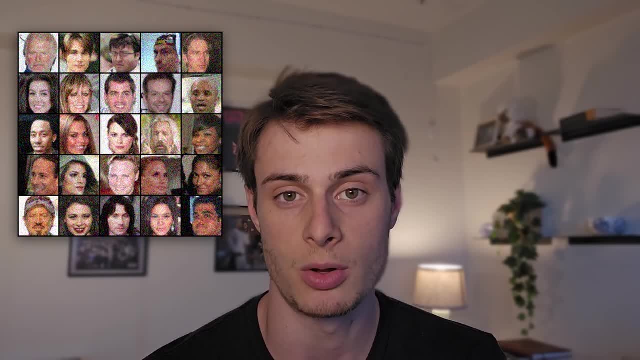 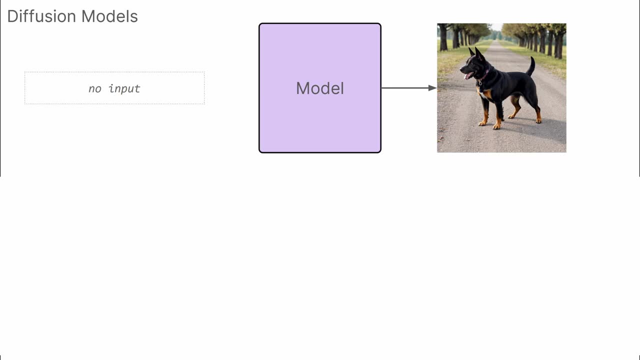 on what's called diffusion models, which generate images from pure Gaussian noise. One limitation of diffusion models is that they just generate any image at random without any way to control the process. Text-to-image models, on the other hand, add the modality of text to guide the image generation process. 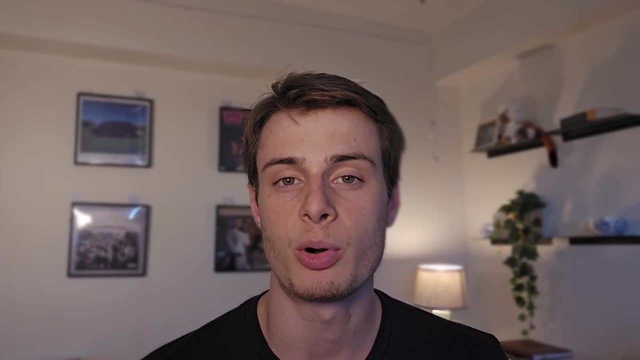 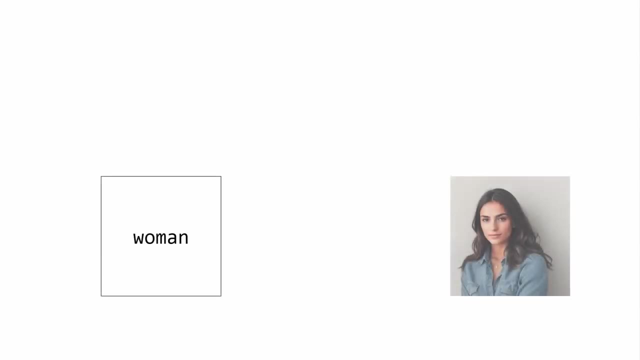 To understand how these models work with both text and images, it's important to first see that both modalities can represent the same semantic concept. In other words, when we see the word woman and we see an image of a woman, we understand that these are just. 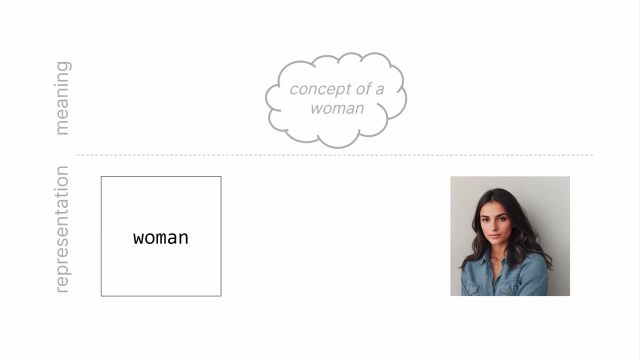 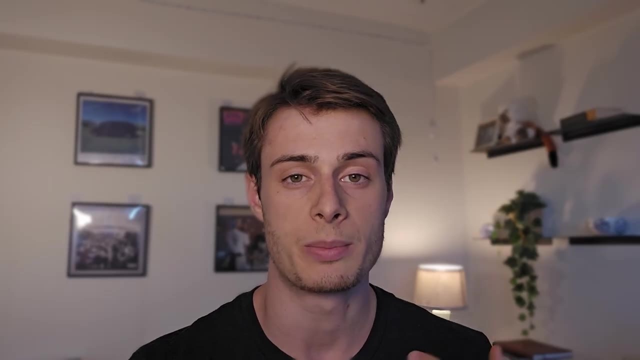 two representations of the same underlying meaning. One is the concept of a woman itself, one is a visual representation and one is a textual representation. Rather than working with these representations themselves, a multimodal AI model will often work with the meaning directly. Multimodal models use 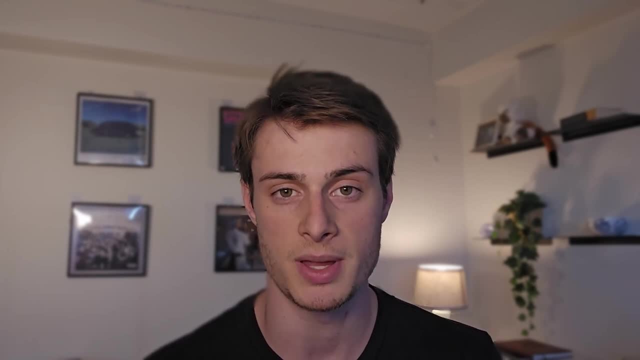 embedding models to convert text and images to vectors that capture their meaning. To learn more about how and why this works, you can check out our video on word embeddings. The relevant question for us is: how are these embedding models trained? There's no single answer to this question, but a model like DALI 2,, for example, actually uses 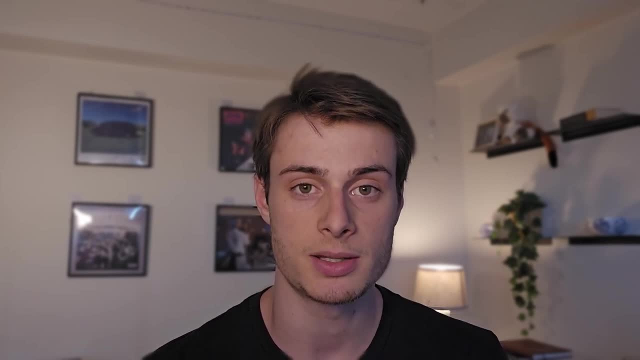 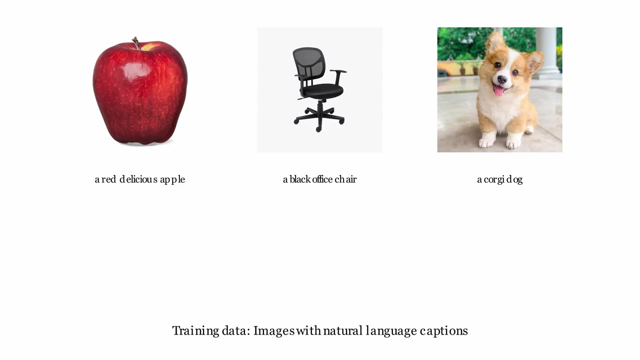 a model called CLIP to train these embedders and therefore learn this meaning space. Let's take a look at how CLIP is trained now. Since our goal is to learn how images and text relate to the same concept, we start with a dataset of images and their captions. 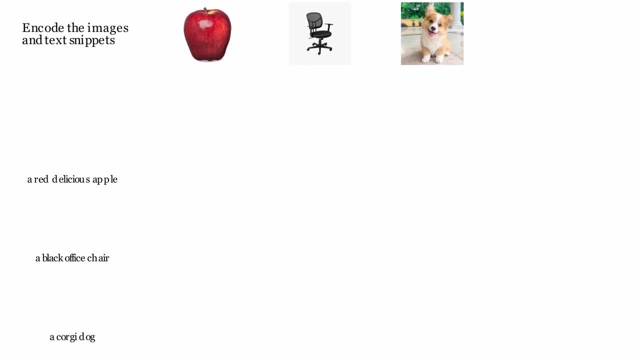 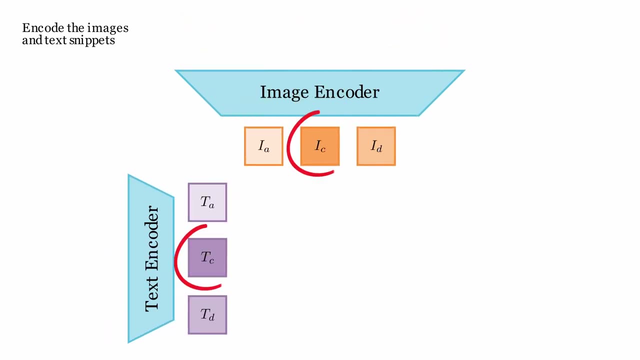 For every pair we encode the text and image using their respective encoder, so we're left with a pair of vectors for each image-caption pair. In our case, we have a pair of vectors for an apple, for a chair and for a dog. 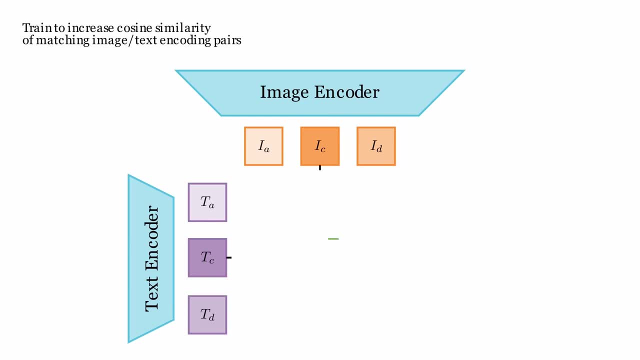 We then train by maxing the cosine similarity of these pairs. The cosine similarity is a distance metric for vector spaces that measures the angle between vectors. By maximizing this similarity, we are pointing the text and image vectors for the same concept in the same direction, giving this direction meaning in the space. 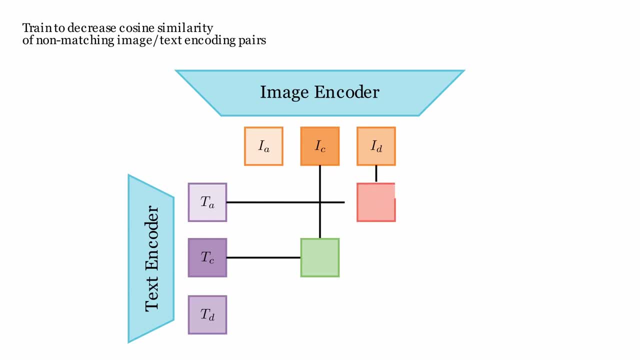 Similarly, we train to minimize the cosine similarity of text and image vectors for two different concepts And we repeat this process for every combination of text and image vector in the batch. In this way, we'll train the encoders to map both text and images to the 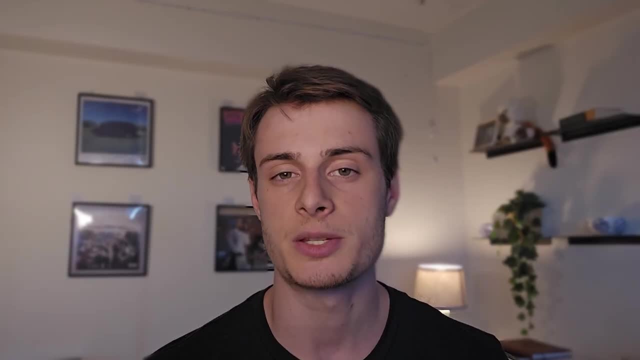 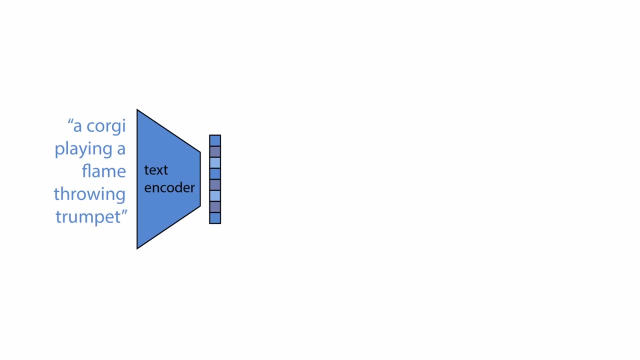 same space in such a way that their meaning is preserved. The learning of the space lies at the end of the process, so we can see how it works in this instance. To generate an image, DALL-E 2 will embed the input text into this meaning space. 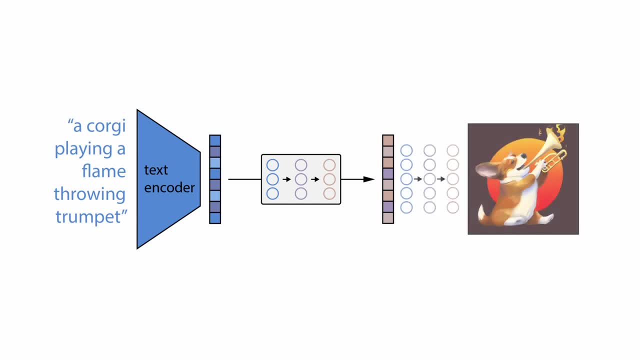 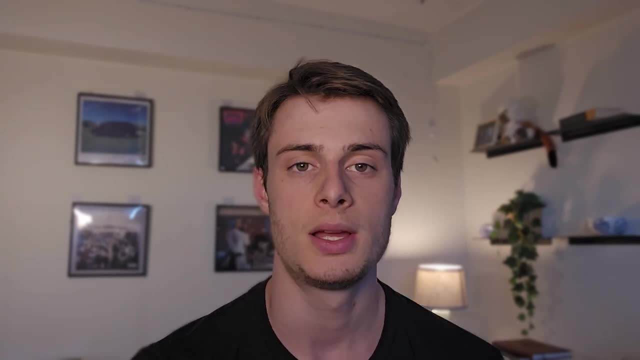 map the meaning textual vector to a visual meaning vector and then decode this visual meaning vector into an image. How this actually works in practice is by conditioning the diffusion model which generates the image. This gets a little complicated, but diffusion models use what are called u-nets to iteratively denoise a Gaussian input into an image. 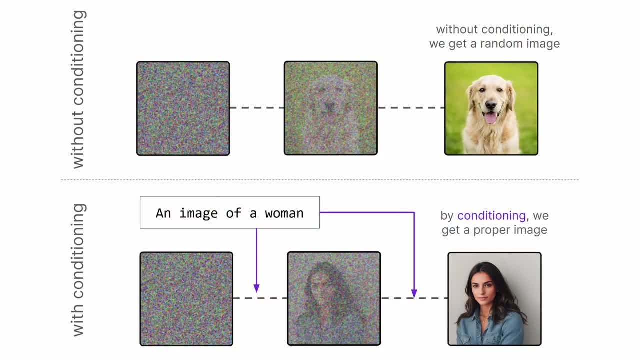 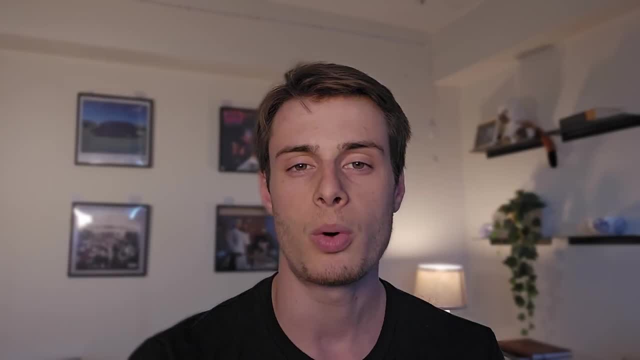 and the meaning vector is used to condition this process to generate a specific image. You can read our article on building your own text-to-image model if you want to actually see how this works under the hood. But what about models that can both input and output multiple? 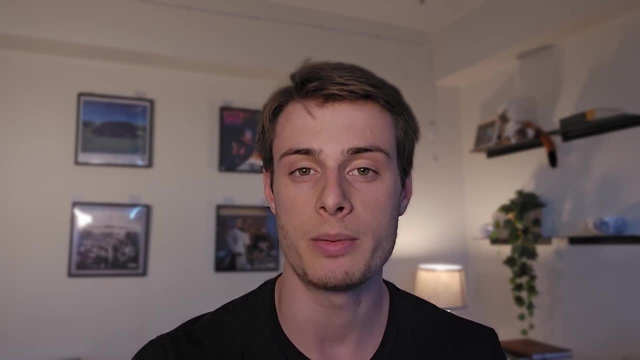 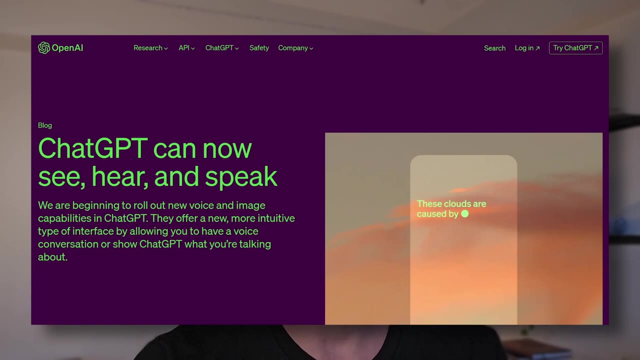 modalities like ChatGPT Text-to-image models only handle one modality at each end of the model: text on the input and images on the output. On the other hand, ChatGPT can now accept images, text and audio and generate images, text and audio. This ability actually leads to an 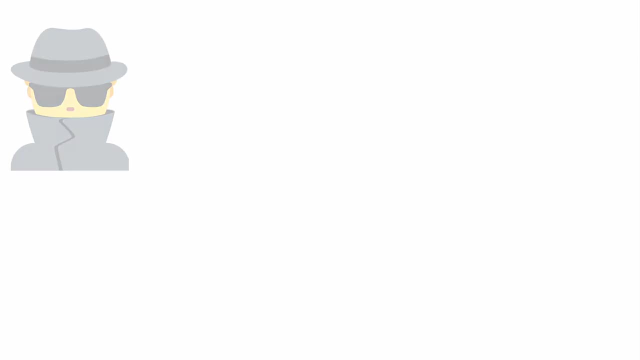 issue that may not be immediately obvious. For example, imagine a detective who describes a crime and then asks ChatGPT to paint me a picture of a man who would commit such a crime. What is the detective asking the model to do? Is he asking the model to metaphorically paint a? 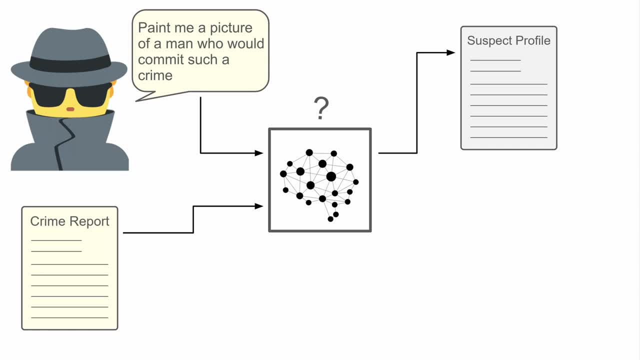 picture of such a man, like his backstory, his motives, etc. Or is he asking the model to literally paint the picture of a man that is, a literal image of his face, perhaps using details from witness reports A priori? the model really has no way to know and in fact humans would give. 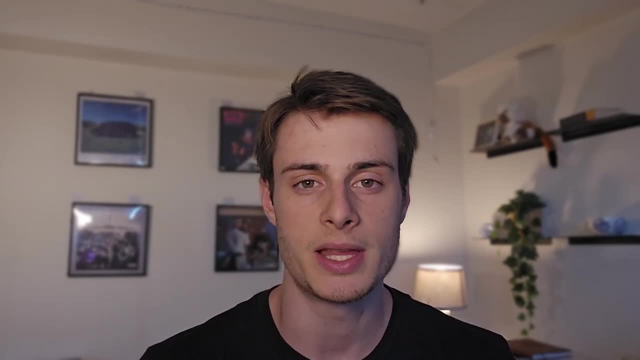 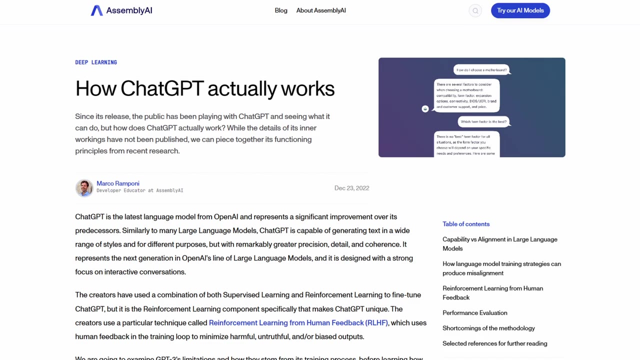 different responses to this same question. The fundamental thing to note here is that when somebody says ChatGPT, he's actually referring to two distinct things. First there's the LLM ChatGPT, which is just GPT with RLHF fine-tuning, and then there's the UI ChatGPT, which is the web.